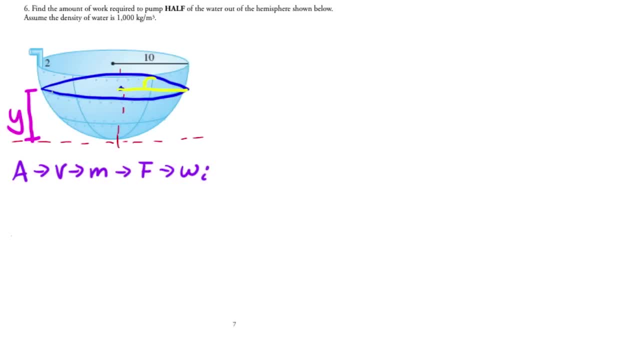 out Okay, so let's start off with the area. So the area of the slab is – I'm going to go through the area of the slab. So the area of the slab is equal to pi r squared. obviously, Now r here. I need to figure out a way to find it. So notice that the distance from 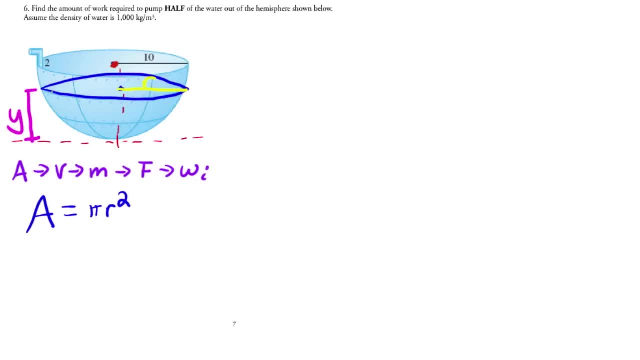 the center of the hemisphere to any part outside, on the edge I mean, is going to be equal to 10 – the radius 10.. So the distance from here to here, that's equal to 10.. And also from the center to the very bottom, that's also 10.. So that means that this guy 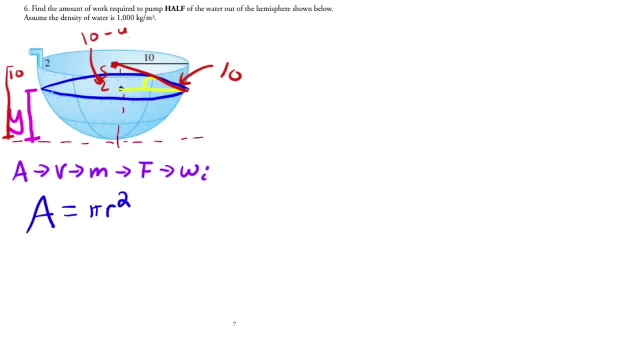 right here. that's equal to 10 minus y. So then what that means is that r is equal to the square root of 10 squared, or 100, minus 10 minus y squared. Okay, So the area of that slab is going to equal to pi times this guy squared, which. 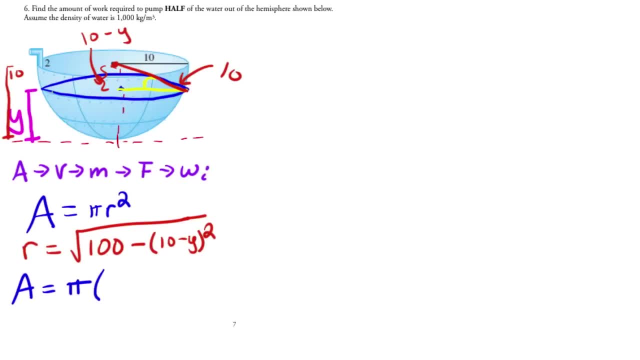 is going to be 100 minus – I'm going to expand the 10 minus y squared, So 100 minus 10 squared is 100.. Minus 20. And so x squared is less than or equal to 1, minus 10.. And so x squared is less than. 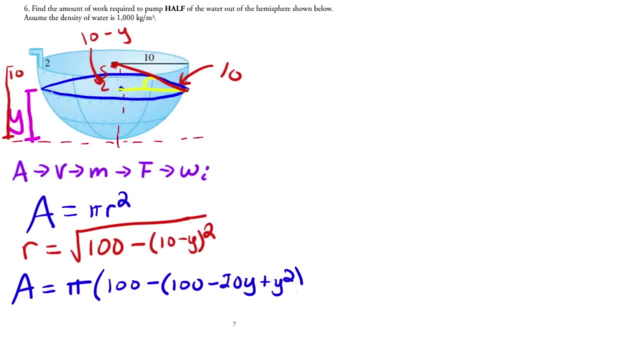 y squared. So minus 10 done, plus y squared. Contrary to that, minus 2 is minus 7 and I搞 20y and then plus y squared. Okay. so then the area of the slab is pi times 100 minus 100. So this is just equal to positive 20y minus y squared. 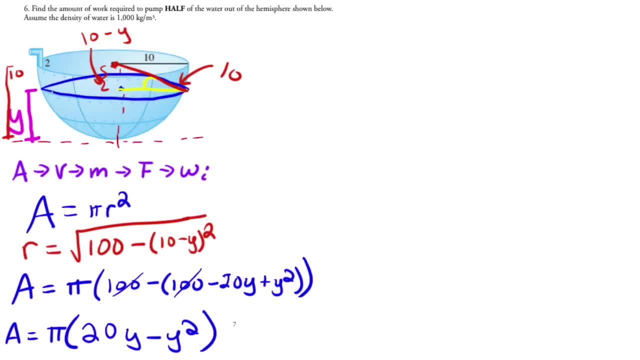 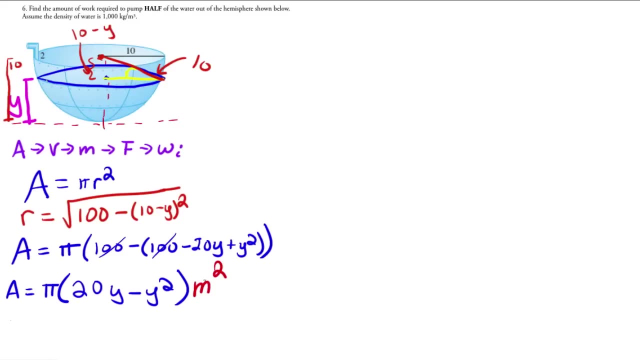 Okay, and so then this is in units of square meters. Let me write this here. So the work for the slab, the work to get the slab out, is going to be pi times 100.. times 20y minus y squared meters squared, And then I'm going to multiply that times, I'm going to remove the parentheses, So just delta y meters, which is going to give me volume, And then multiply that by the density. 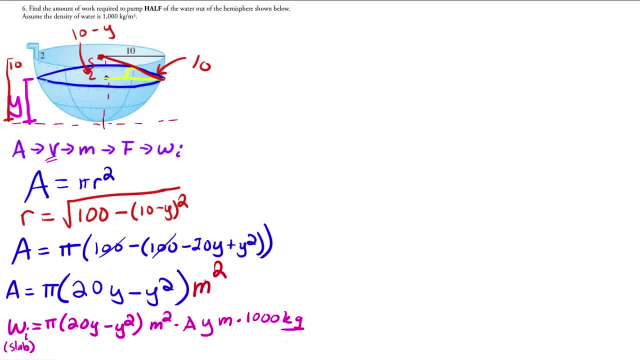 which is 1000 kilograms per meter cubed, which is going to give me the mass. times, 9.8 meters per second squared, which is going to give me the force, And then times. now, this one is critical. This is the distance that this slab needs to travel, to go. 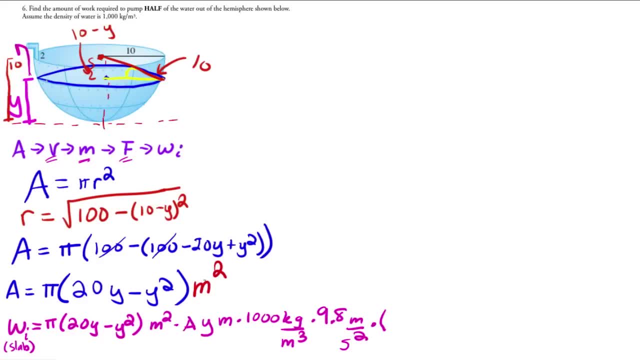 out of the tank from where it is outside. So this guy is located at y, So then the distance that it needs to travel is going to be 12 minus y meters. So just to make sure that that's clear, let's just kind of pretend that. 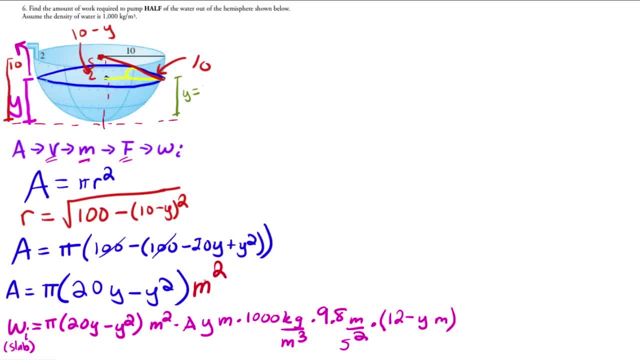 this slab is located at y equals to, let's just say, four, for example. So if this guy is at y equals to four, then what's going to happen is this guy is going to need to travel another six to get to the top, because it's 10 from here to here, So it's going to need to go six plus another two, So that's eight. So 12 minus four is going to be 12.. 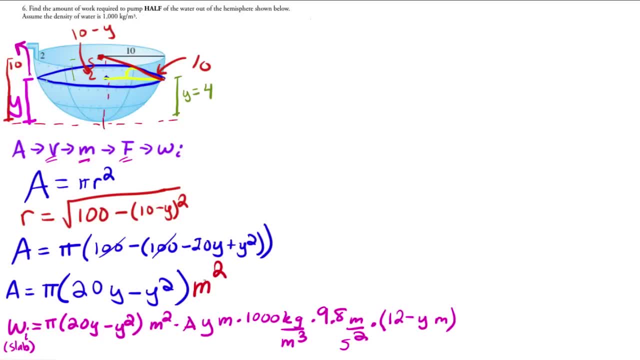 So that works. So that's the explanation for that guy. Now, depending on your setup, this might have been different because of where you put your axis, but it would still be correct, as long as these match up Where you place your axis, the distance. this has to be the distance that it needs to go. 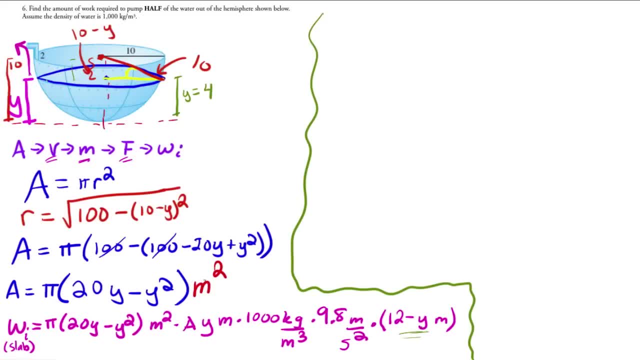 out, and your limits of integration should also match. But anyways, if I simplify this, I'm going to get 9800 pi times 20y minus y, squared times 12 minus y, So then the total work would be the integral. 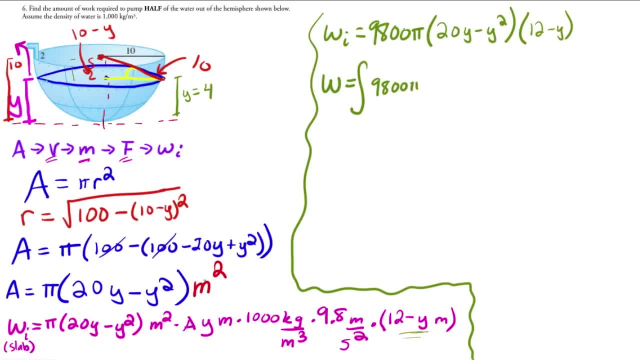 The integral of this guy: 9800 pi times 20y minus y, squared times 12 minus y. with respect to y: Oh, I forgot my delta y here. remember that turns to dy as delta y goes to zero. Now this is important, since we're pumping half of the water out of the tank. the limits: 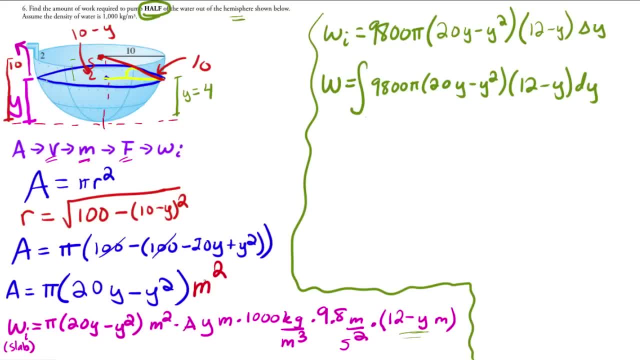 of integration have to remain the same. So this is going to represent what y is going to go from and to. So, since we want to pump half of the water out and I have my setup here, as my distance that the slab of water needs to travel is 12 minus y, then what it's going to do is 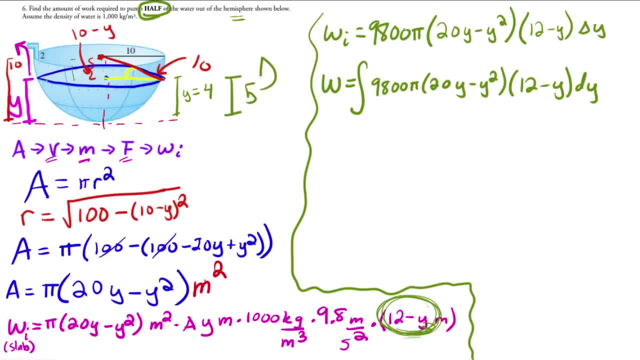 it's going to go from 5 all the way up to 10.. Okay, So that's that. Okay, So that's going to go from 5 all the way up to 10.. So, basically, my first slab of water, for example, is when y is equal to 5.. 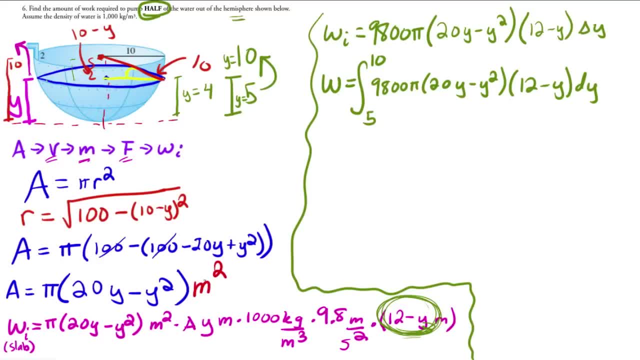 So that one needs to travel 12 minus 5 or 7.. So the one, the very first one, needs to go a total of 7 meters to get out, which makes sense, because it needs to go 5 plus another 2..